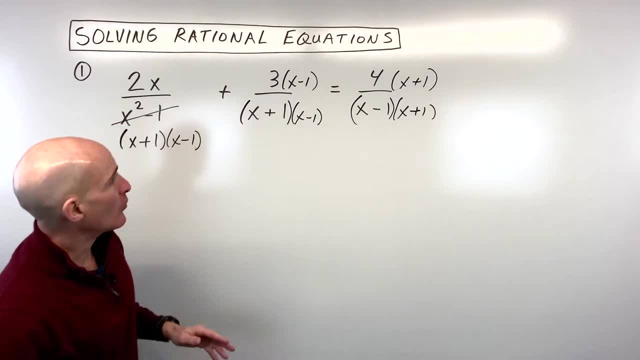 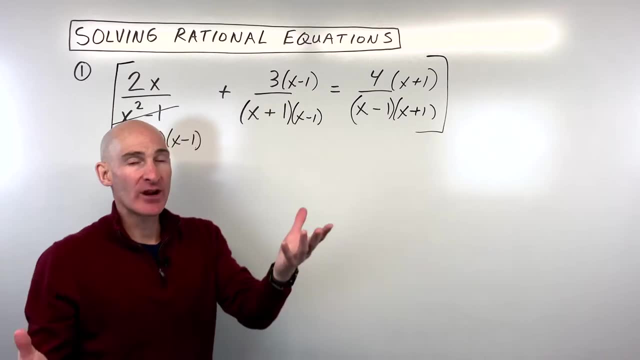 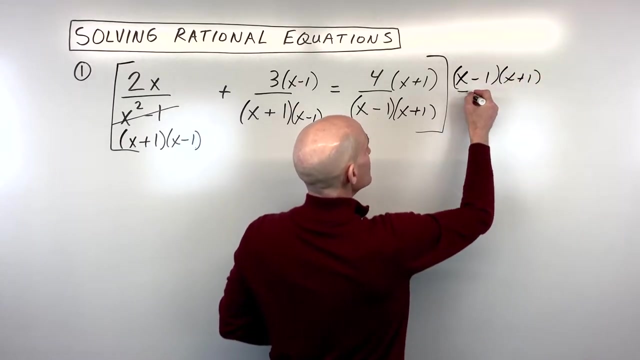 denominator for all three of these, these fractions, and what we're going to do now is we're going to clear the denominators, meaning we're going to multiply this whole equation, both the left side and the right side, by this common denominator, which is x minus one. x plus one. You can think. 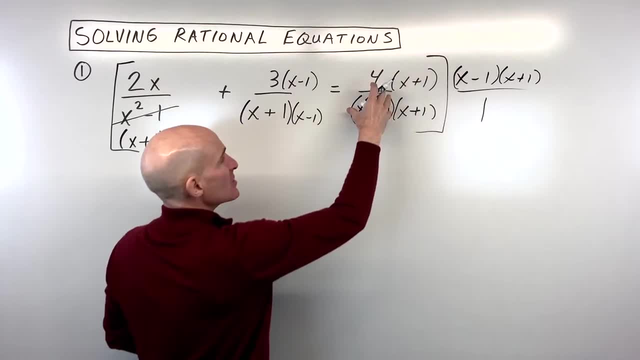 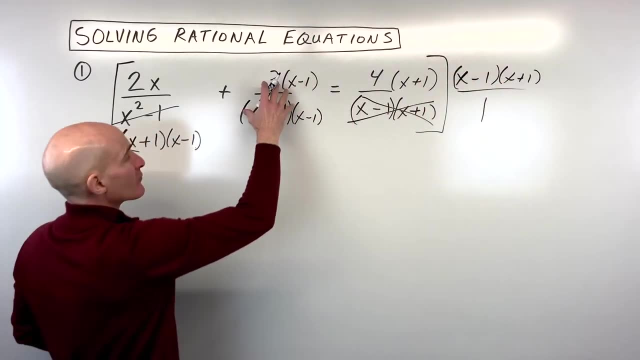 of this as being over one. Now, if you were to do that over the denominator, you would have to do the same thing over and over again. So if I'm going to distribute this to this fraction here, you can see that x minus one, x plus one would cancel out this denominator If you distribute it to this. 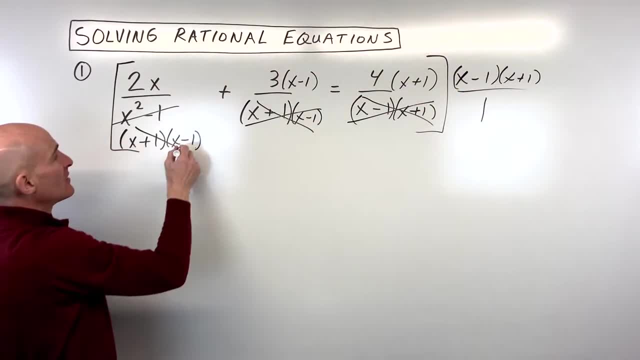 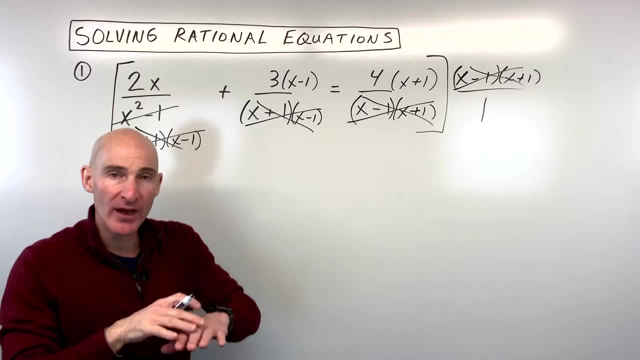 fraction here you can see it's going to cancel out this denominator and if you distribute it to this fraction here cancels out this denominator. So what happens is you're clearing the denominators by multiplying through that equation by that common denominator, You're keeping the equation. balanced, because you're doing it to both the left and the right sides. And so then now what this does. it makes it a lot easier If you're going to distribute it to the left and the right sides, so you don't have to do that. 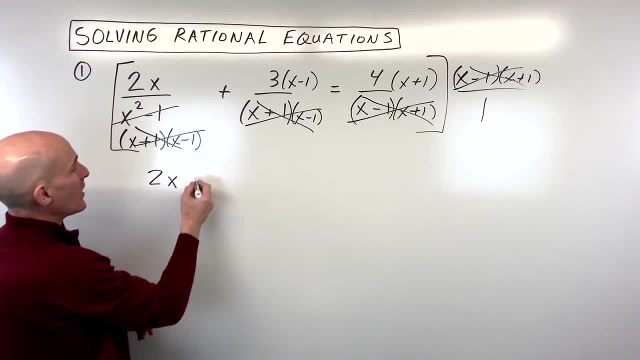 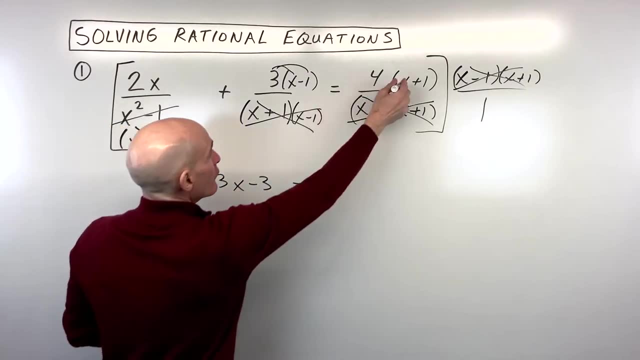 easier to solve because we're just left with the numerator here, which is 2x plus 3x minus 3 equals 4x plus 4.. Okay, so now let's just go ahead and solve. It's just like a normal. 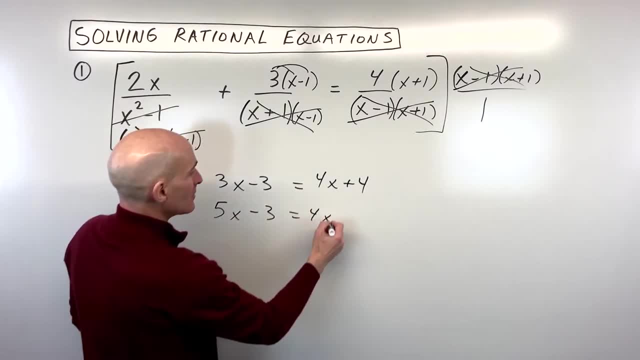 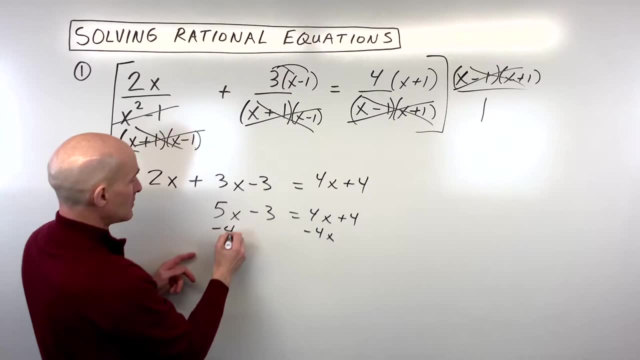 kind of easy algebra equation, right? And so what we're going to do is we're going to subtract 4x from both sides, add 3 to both sides, and now you can see this is coming out to: 1x is equal to 7.. And what you want to do before you call it a day on that problem? 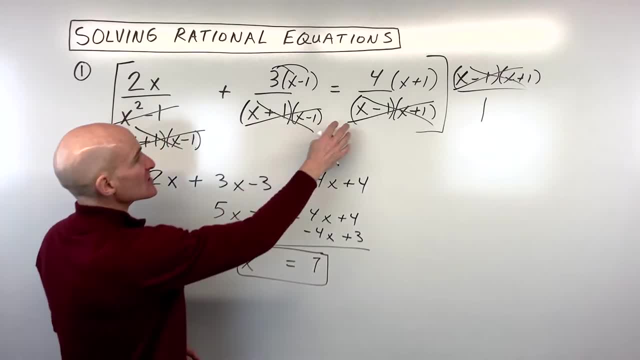 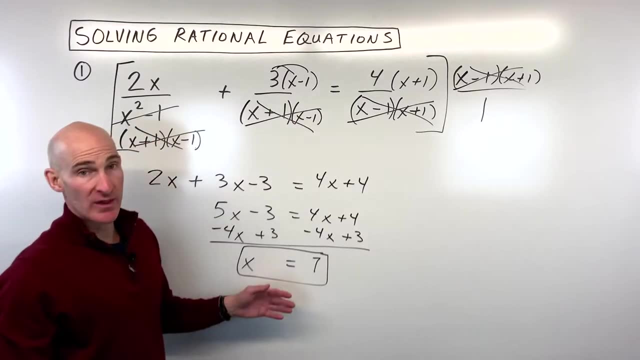 is. you want to take that 7 and you want to go back and look at the denominators and see if it makes any of the denominators equal to 0. If it does, that's called an extraneous solution. It's a false answer and you would then say that there's no solution. But in 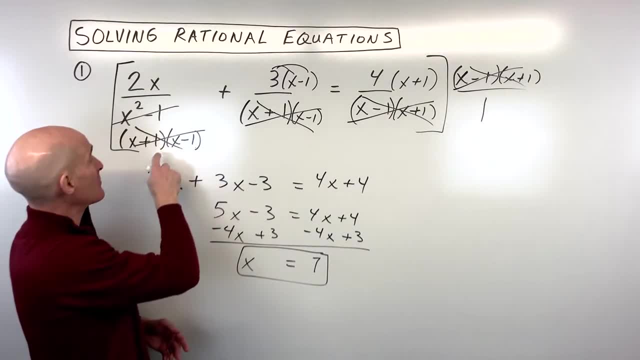 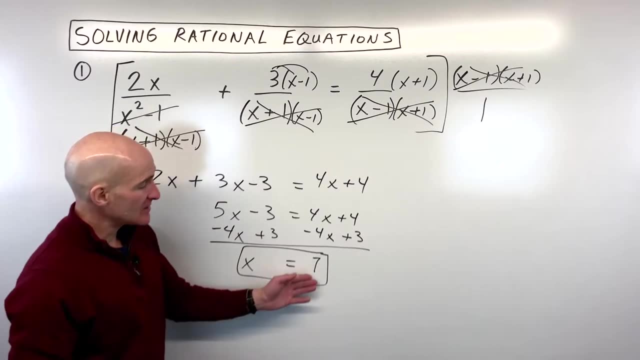 this case. we just solved it. We just don't want the denominator, the x value, to come out to negative 1 or positive 1, because that would make the factors in the denominator equal to 0, and you can't divide by 0. That's undefined In this case 7, that's not going to make the denominator 0, so this: 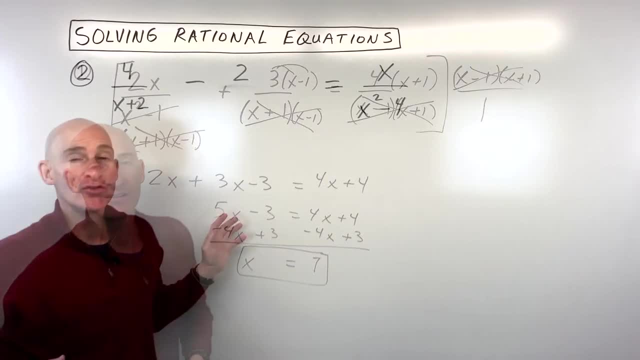 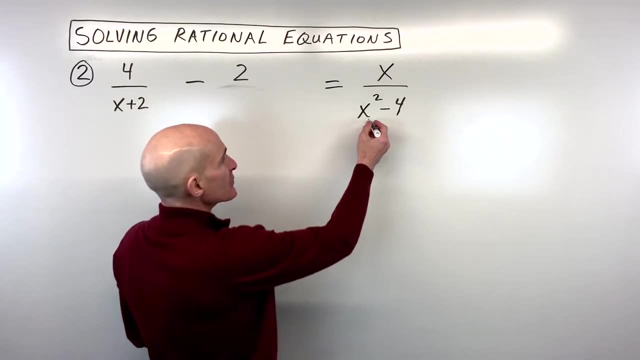 is a good answer. Let's take a look at another example. See if you can do number 2 on your own. If I was going to do this, what I would do is I'd factor the denominators as much as I can first. This is the difference of two squares: x plus 2 times x minus 2.. This 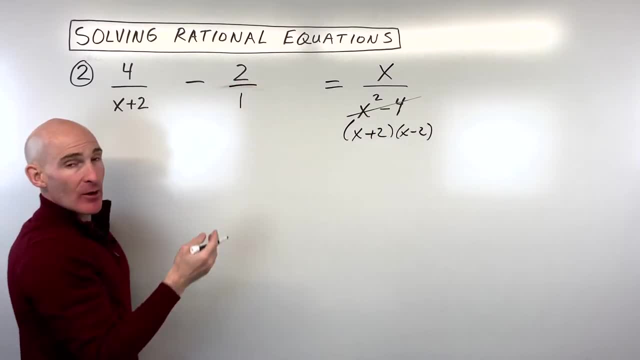 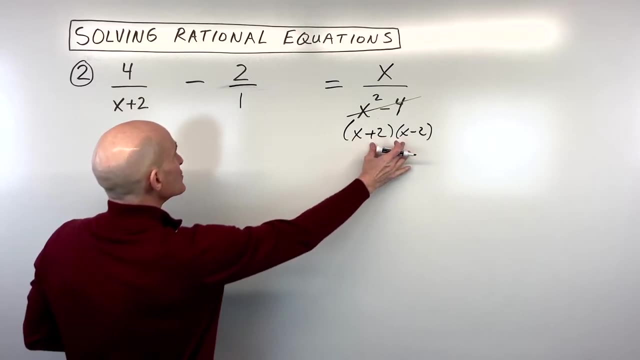 one you can think of as a fraction by putting it over 1, because anything divided by 1 is itself. So now, when we look at all these denominators, we want to get a common denominator right. So it looks like we've got an x plus 2, x minus 2.. We only have an x plus 2 here, so 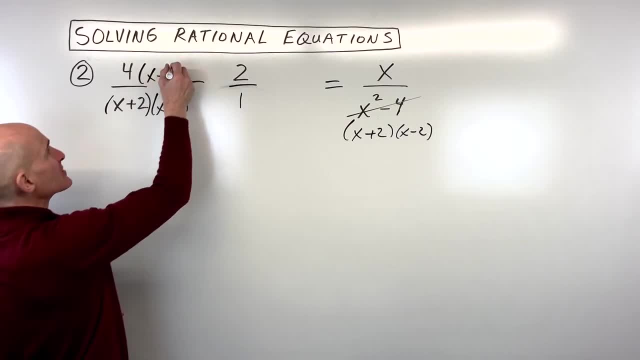 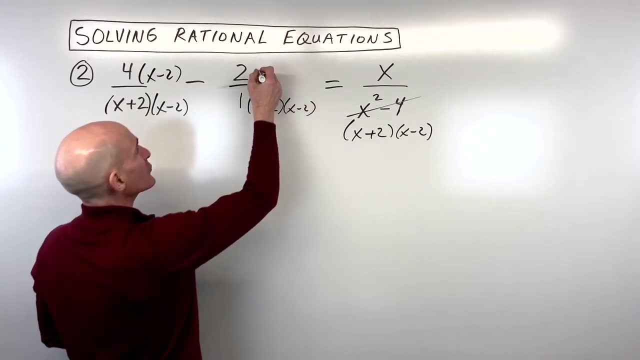 that means we need an x minus 2, so I'll multiply that to the numerator and denominator. Here we're missing both an x plus 2 and an x minus 2, so we're going to have to multiply those both to the numerator and denominator. Now we can see that we have a common denominator. 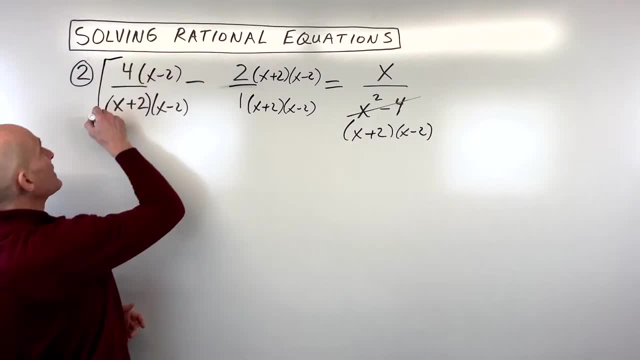 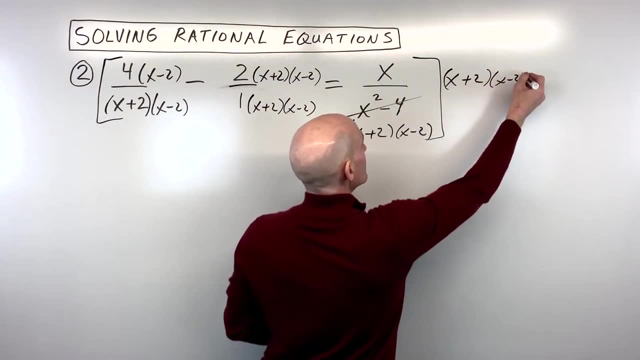 for all three fractions. so what we're going to do is we're going to multiply the left side and the right side by that common denominator, x plus 2, x minus 2.. And you're keeping it balanced because you're doing it to both sides. I just like to think about it as multiplying. 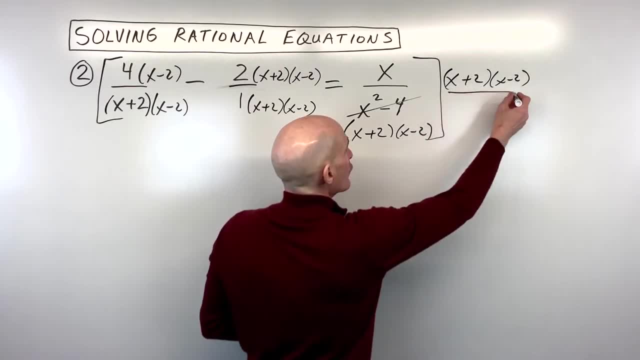 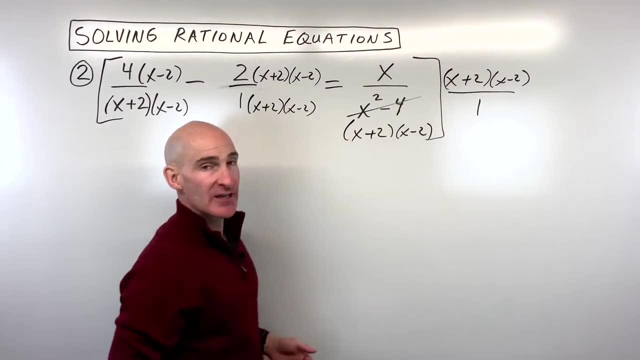 the entire equation by that And again you can think of this as being over 1, so what happens when you multiply it to this fraction? here the x plus 2 and x minus 2 in the numerator cancel with the x plus 2, x minus 2 in the denominator. Same thing here. same thing here. 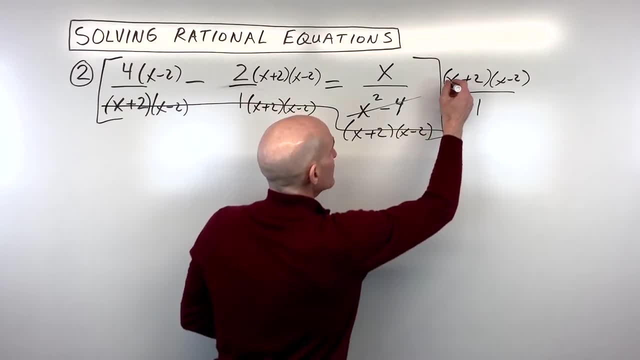 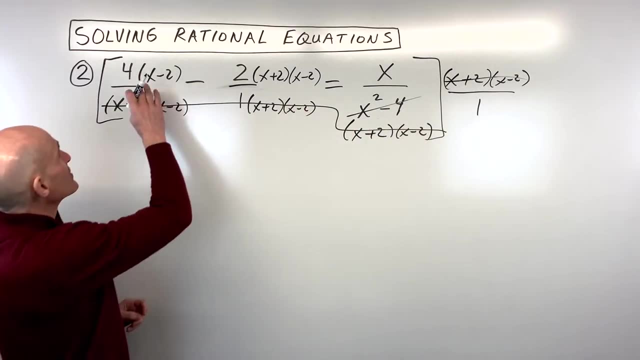 What ends up happening is we end up clearing the denominators- and that's a nice feeling, right- Just crossing out all those fractions. We just have to deal with the numerators now, right, So let's go ahead and do that. So we're just going to simplify. We've got 4x minus. 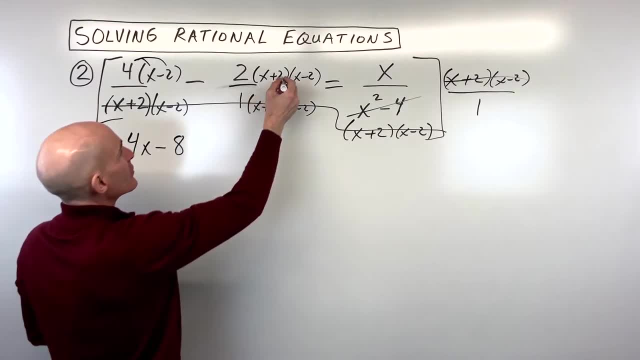 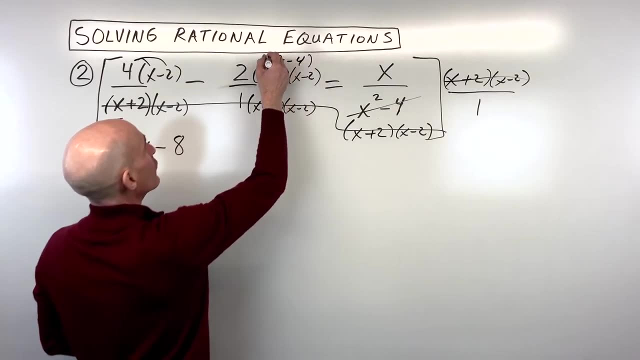 8.. Okay, and then here, if we multiply these together, remember x plus 2 times x minus 2, that was this x squared minus 4, so I'm going to write this as x squared minus 4.. And this minus 2 I'm going to think of as a negative 2 that I'm distributing into the 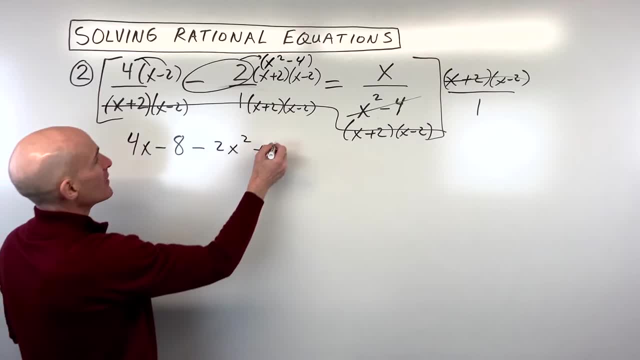 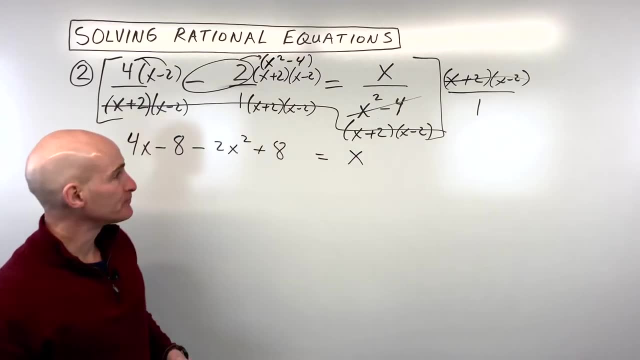 parentheses there. So that's going to give us negative. 2x squared plus 8 equals x. Okay, now we have a little bit simpler equation to work with, right? So what I'm going to do is I'm going to get everything on one side of the equation and set it equal to 0.. So if I do that, let's 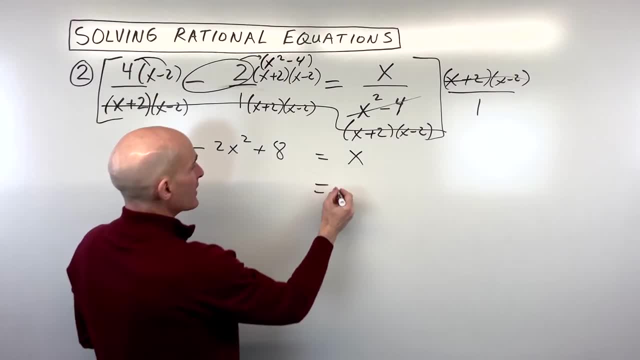 see I've got- let me add the negative- 2x squared to the right, so that would give us positive 2x squared. Let me subtract the 4x, so 1x minus 4x is going to give us negative. 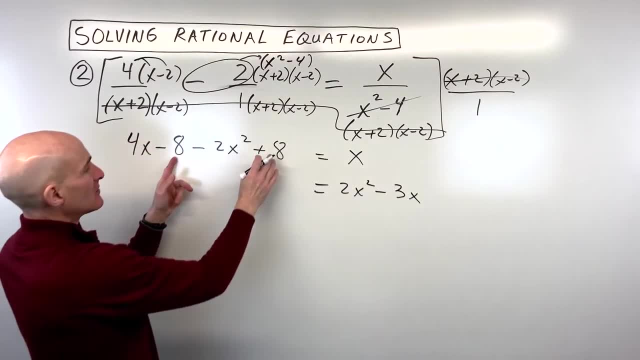 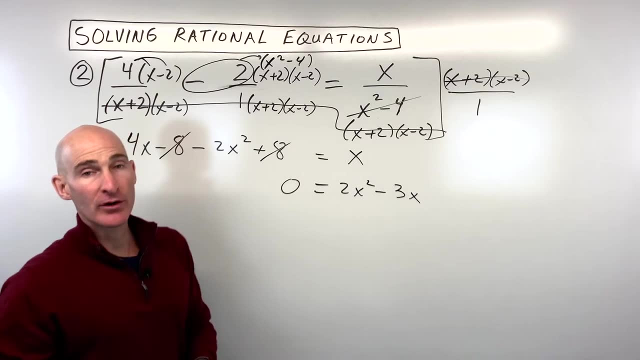 3x, And then here we have negative 8. So I'm going to add 2x squared plus 8, which is actually 0.. Those guys cancel. So now we've got everything on one side, we set it equal to 0, and we're going to factor. So the only 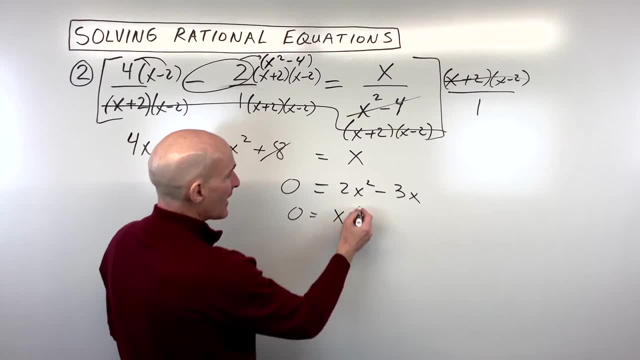 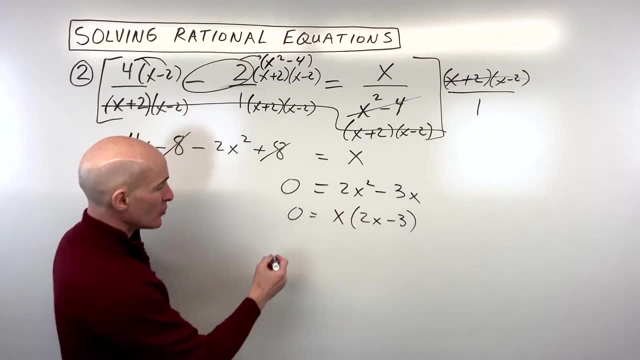 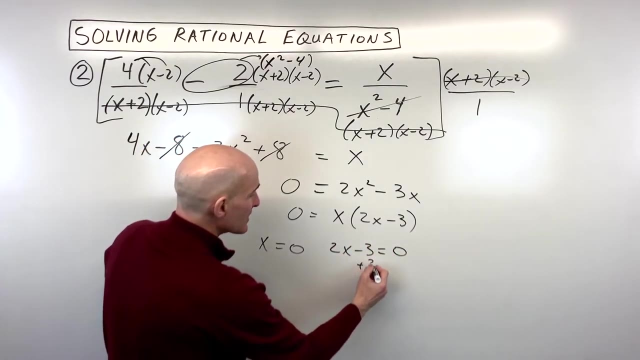 thing we can really factor out here is the greatest common factor of x, which leaves us with 2x minus 3.. When you have it in factored form like this, you can set each group equal to 0,, each factor equal to 0. So x equals 0, and 2x minus 3 equals 0.. Add 3 to both. sides, And then we're going to add 2x squared minus 3.. So we're going to add 2x squared minus 3.. And then we're going to add 2x squared minus 3.. And then we're going to add 2x squared. 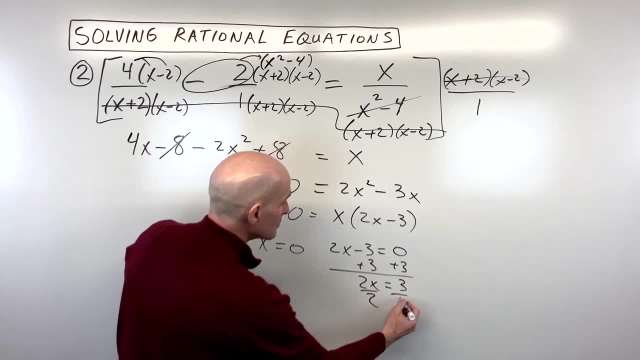 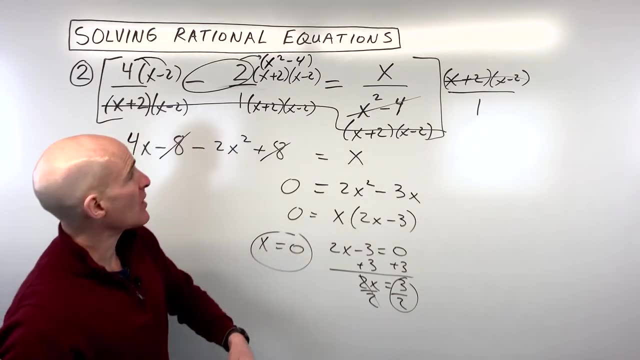 minus 3. And divide by 2.. So you can see that x is coming out to 3 halves or 0.. Now what you want to do, just like the previous problem, is you want to go back and you want to say: hum, does that make my denominator equal to 0?? Well, the only thing that would 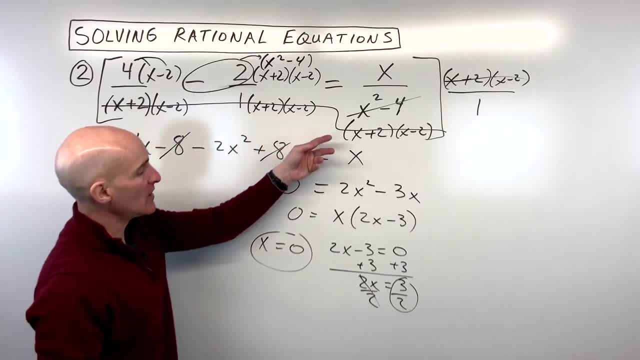 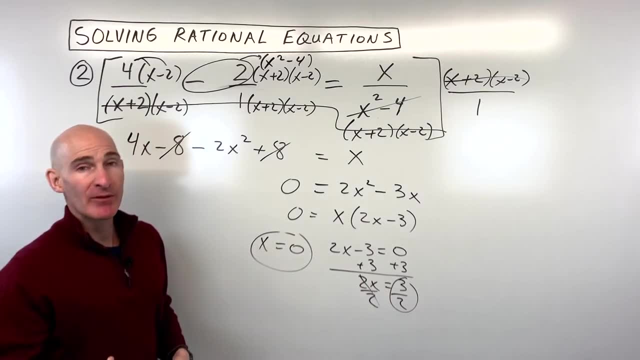 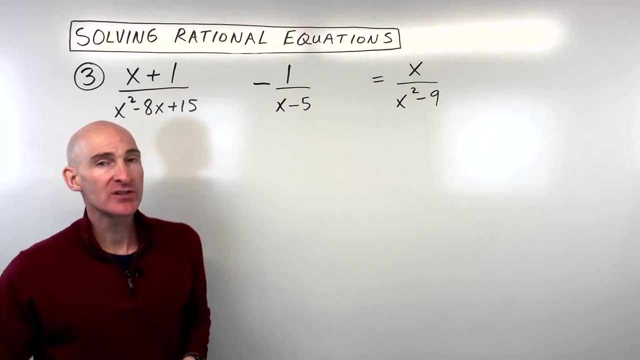 make. the denominator 0 is if x was negative 2 or positive 2.. That's not what we have here. So these are both solutions to this equation, So great job. let's take a look at one more example: me here. I just wanted to mention that I've got a two video courses for sale, an algebra one and an. 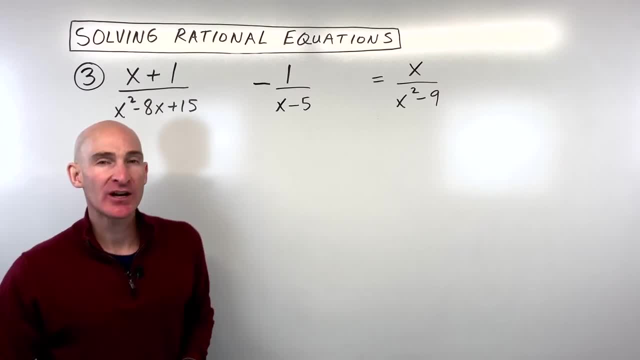 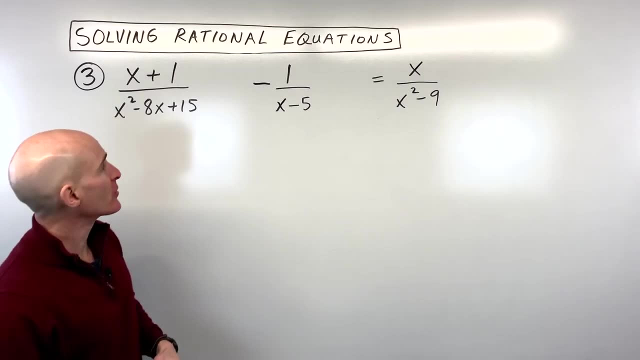 algebra two video course for sale. so if you like the way that I explain things, check out those video courses in the description below. and let's do this last example. see if you can do it on your own, see if you can test yourself here. this one's a challenging one. if I was going to do it, the 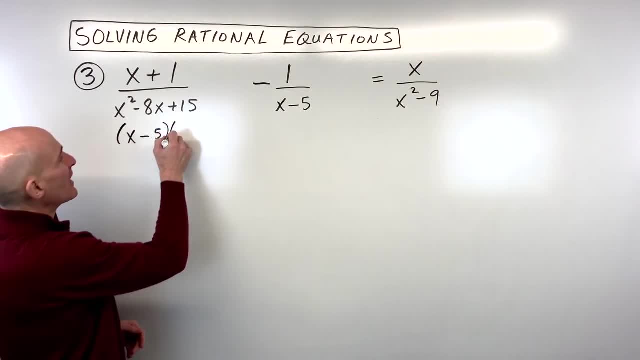 first thing remember is to factor the denominators as much as you can. so in this first one you can see what multiplies to positive 15 but adds to negative 8. that's negative 5 and negative 3. over here it looks like this denominator is already factored and then this one looks like: 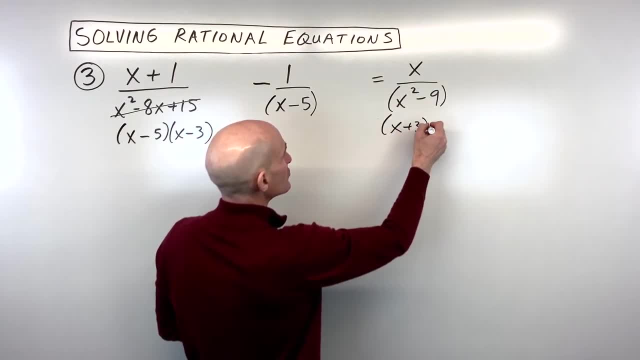 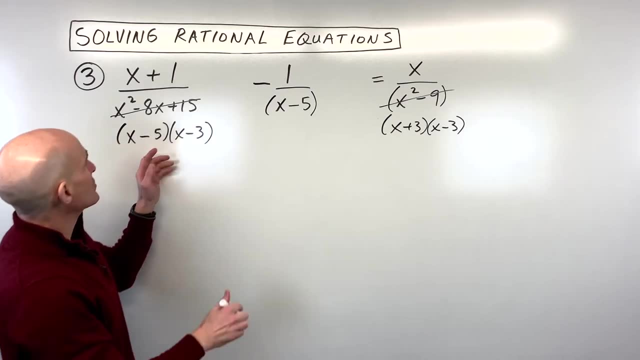 we have a difference of two squares, so that's going to factor to x plus 3 times x minus 3. okay, so now we have to get a common denominator for all three fractions, right? so it looks like we have an x minus 5 here and x minus 5 here. we don't have an x minus 5 here, so let's go ahead. 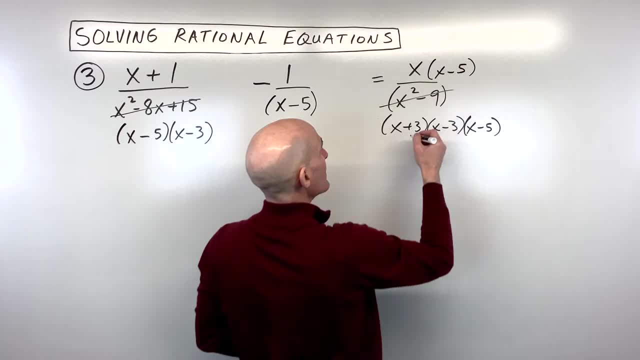 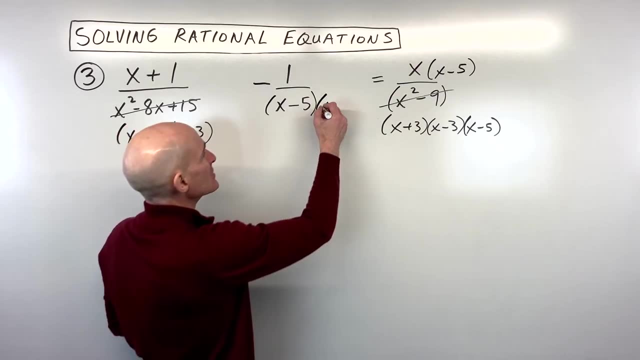 multiply the numerator and denominator by x minus 5. over here we have an x minus 3, here we have an x minus 3. this one doesn't have an x minus 3, so let's multiply the numerator and denominator here by x minus 3. 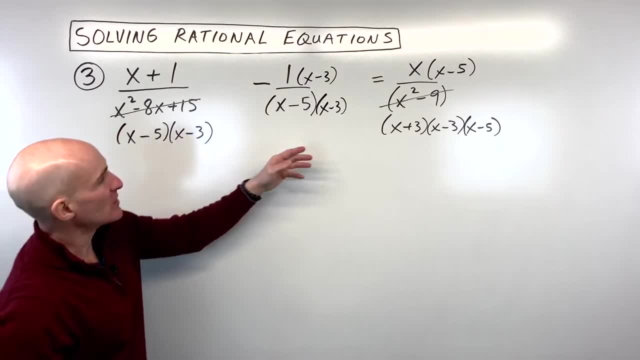 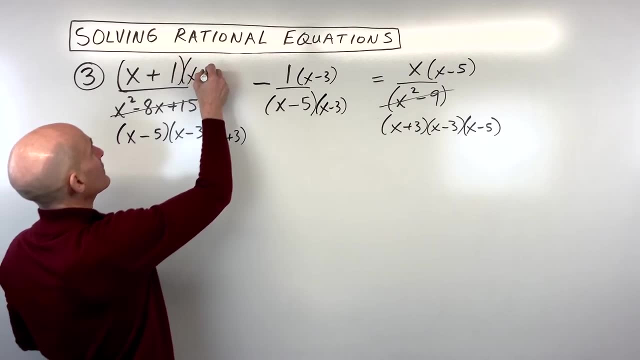 and let's see what else we're missing: an x plus 3. we have an x plus 3 here. we don't have an x plus 3 here, so let's multiply the numerator and denominator by that. this one also doesn't have an x plus 3, so let's multiply the numerator. 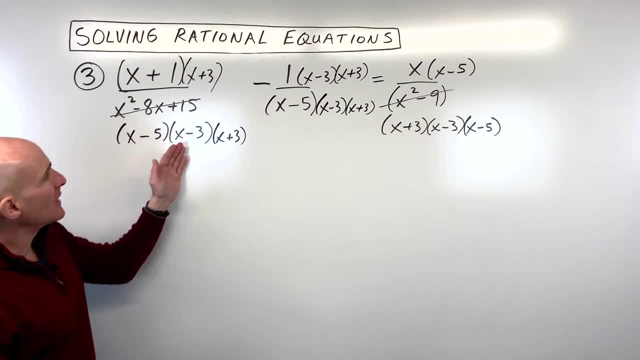 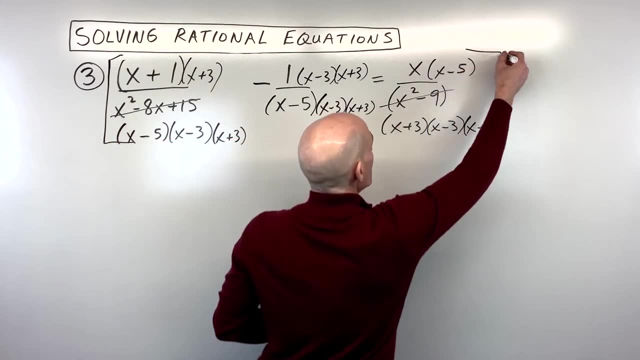 and denominator by x plus 3. now, when we look, it looks like now we have a common denominator for all three fractions. so what we're going to do is we're going to to clear those denominators by multiplying through by our common denominator, which is the x plus 3,. 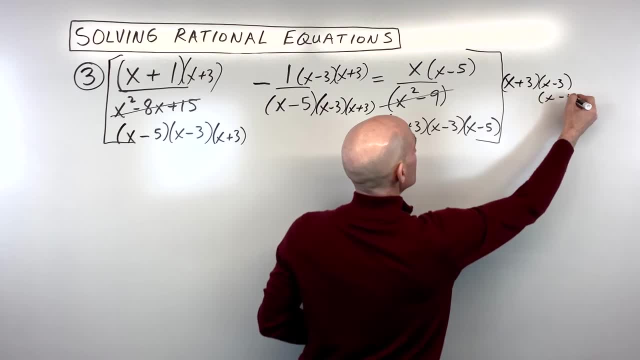 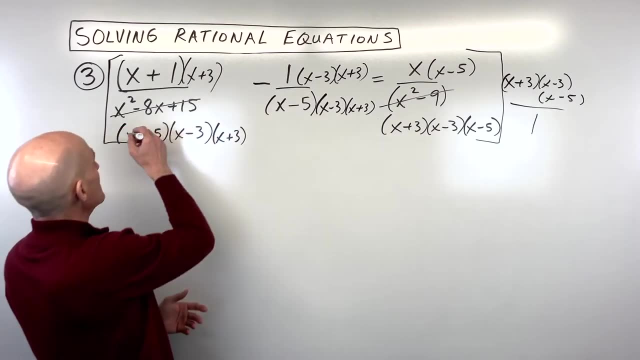 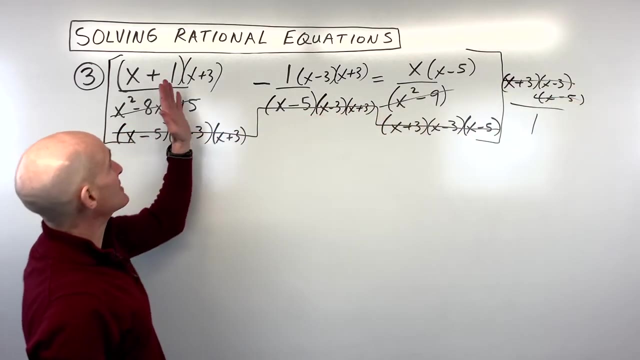 x minus 3, and x minus 5.. And if we do that- remember this is over 1, and distribute to everything left and right side to keep that equation balanced, What that does is it clears the denominators and we've got a much easier equation to solve. We just have these numerators. 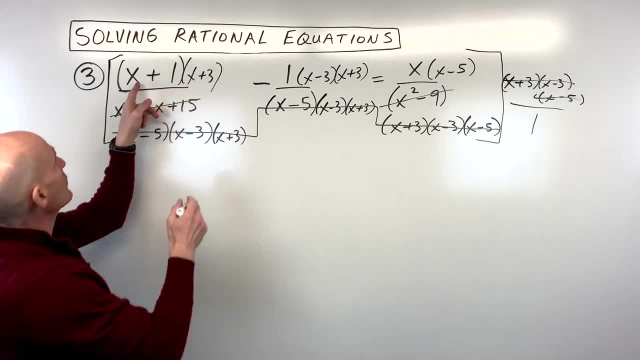 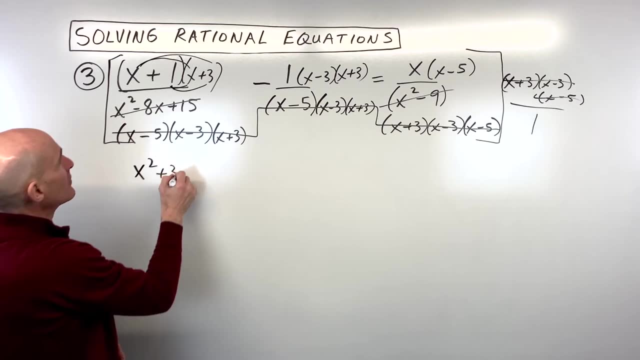 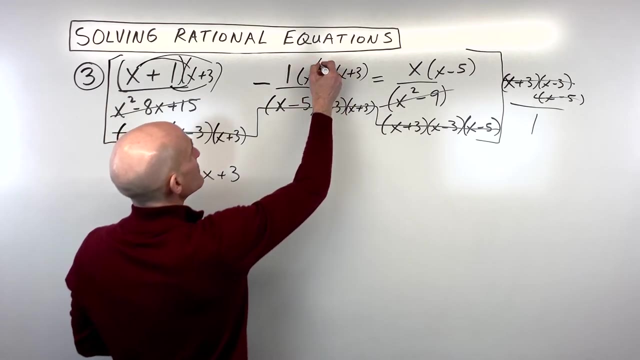 So let's go ahead and simplify the numerators here. what's left? We're going to do the distributive property twice, or FOIL, if you know that method. This is going to come out to x squared plus 3x plus 1x plus 3.. Over here, x minus 3 times x plus 3 comes out to x squared minus 9.. 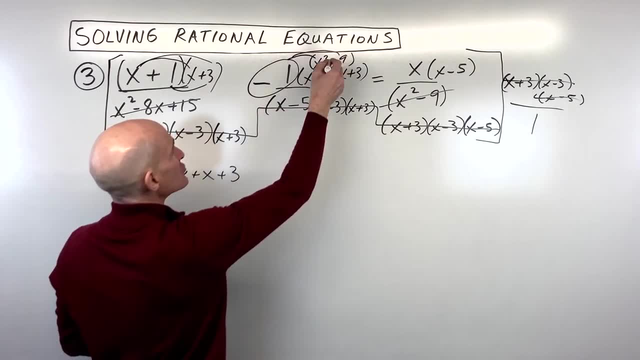 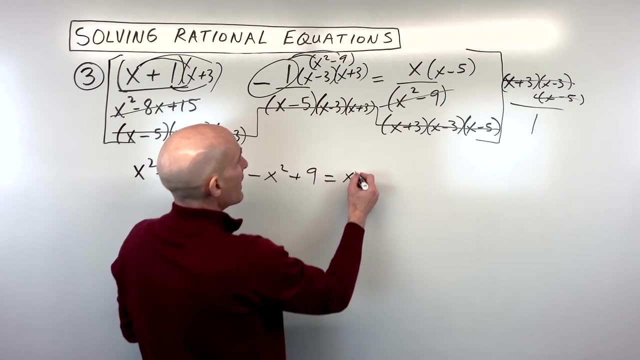 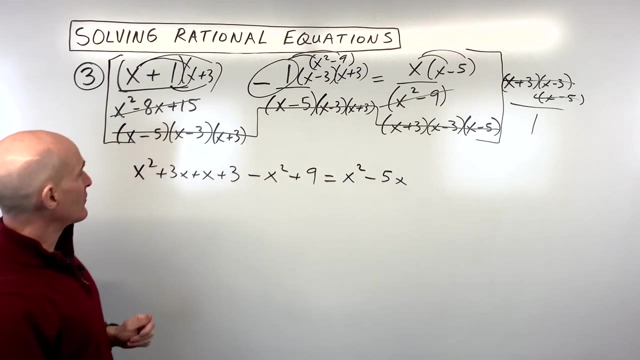 But you see this minus 1? This is like a negative 1 that I'm going to distribute. So that's going to come out to negative x squared plus 9, and then that's equal to x squared minus 5x. Okay, so now we've cleared the denominators. We just have what's left here from the numerators. 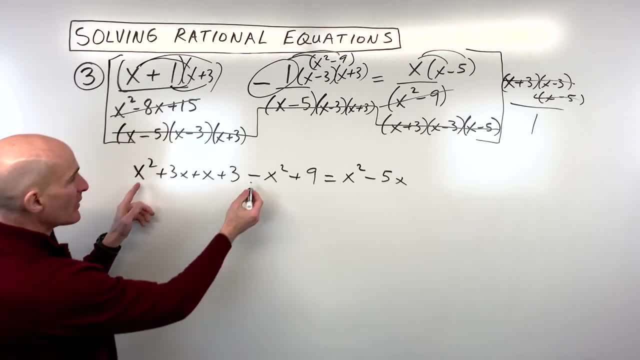 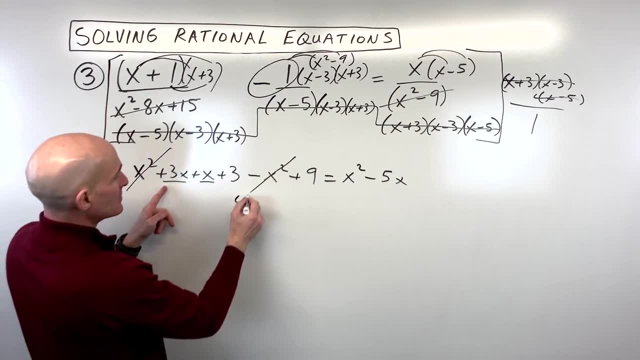 We just have to solve this equation. So let's see what we have here. We have negative x squared and positive x squared. Those cancel. We have: 3x plus 1x is 4x, 3 plus 9 is 12.. 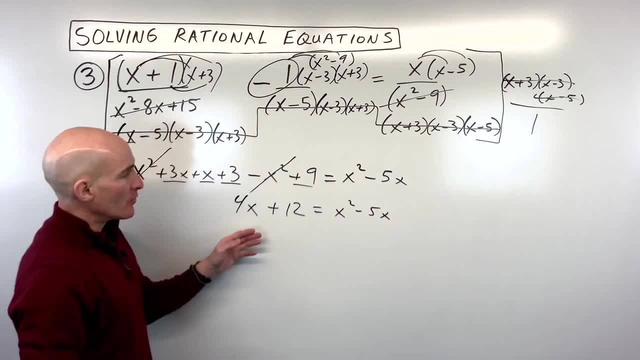 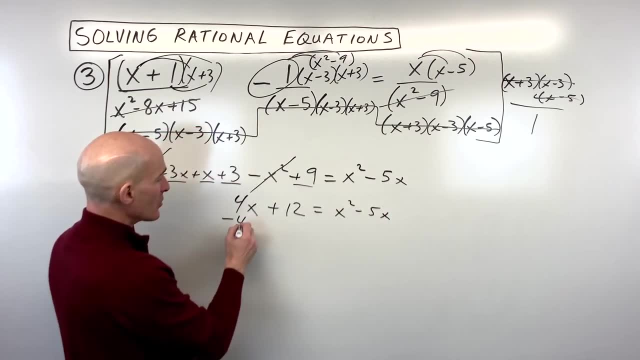 And x squared minus 5x on the right side. So because I've got an x squared term and an x to the first term, what I'm going to do is get everything on one side of the equation and set it to zero. So let's go ahead and subtract the 4x and the 12 from both sides to keep it balanced. 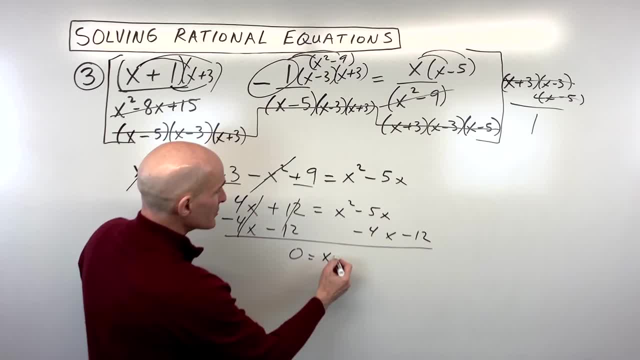 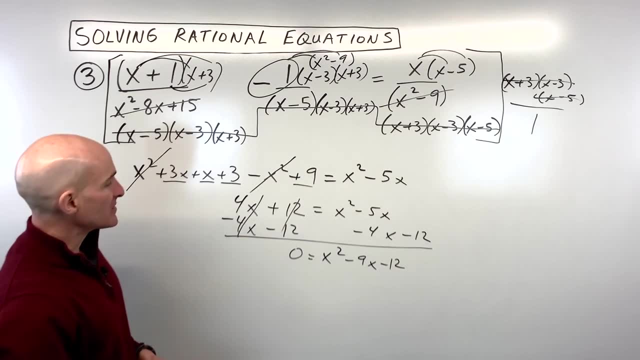 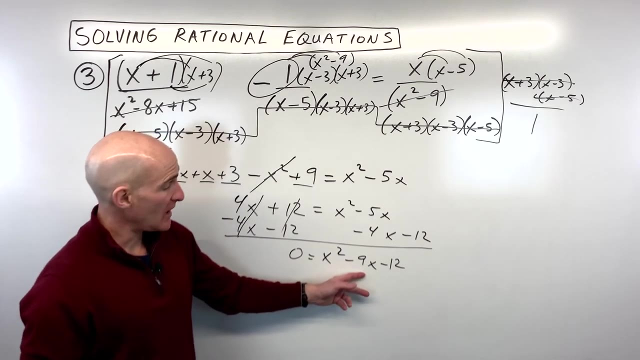 This is going to cancel. We're just going to be left with zero equals x squared minus 9x minus 12.. Okay, now, that's interesting, because what multiplies to negative 12 but adds to negative 9? Well, there really isn't anything. So what we're going to have to do here is we're going to have 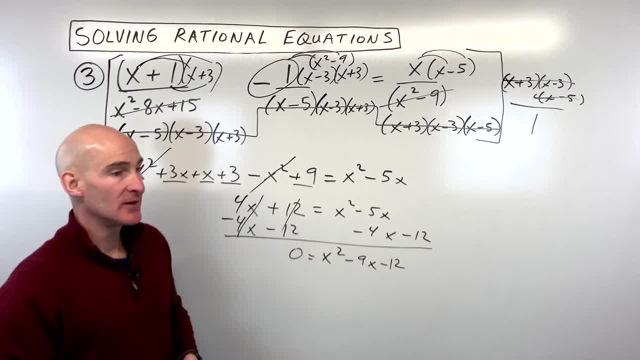 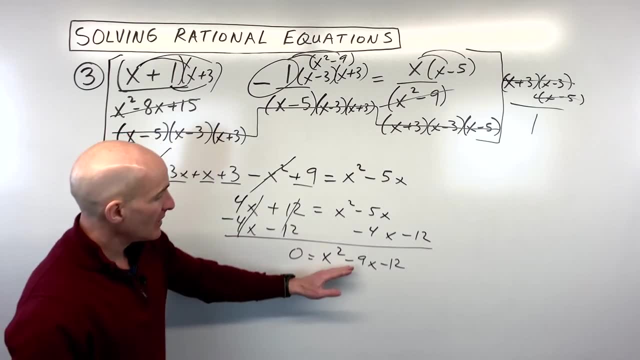 to do the quadratic formula or the completing the square graph, it any of the different methods to solve quadratic equations. I'll just do the quadratic formula. So we've got negative b, which would be the opposite of b, so that'd be positive. 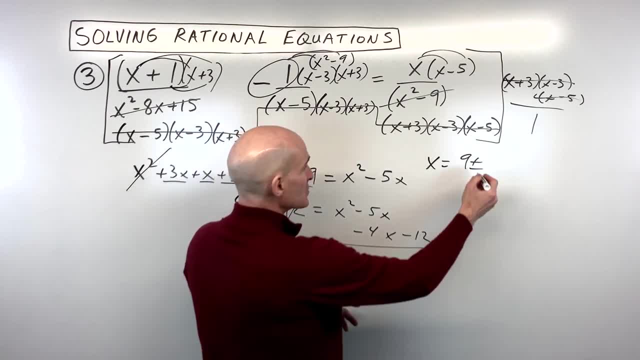 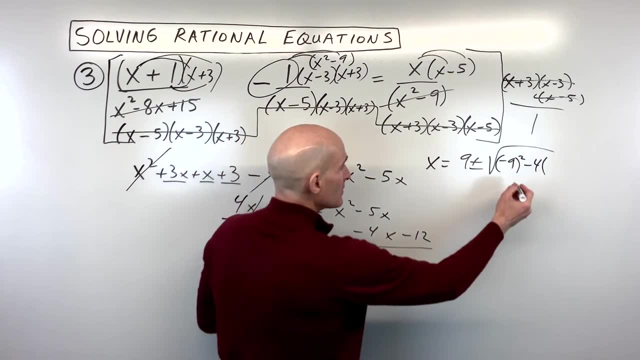 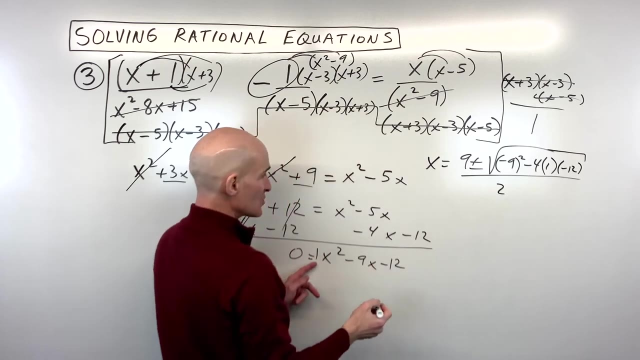 9, plus or minus the square root of b squared, So that's going to be negative 9 squared minus 4 times a, which is 1, times c, which is negative, 12, all divided by 2 times a, which is 1.. 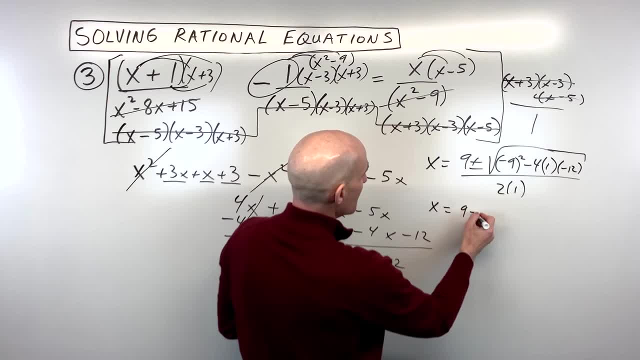 Okay, so you know your quadratic formula. You're going to have to do the quadratic formula. You're going to have to do the quadratic formula. So this is going to come out to, let's see, 9 plus or minus the square root of 81 plus 48,. 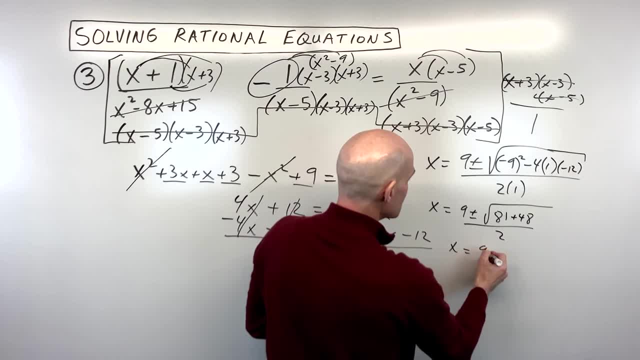 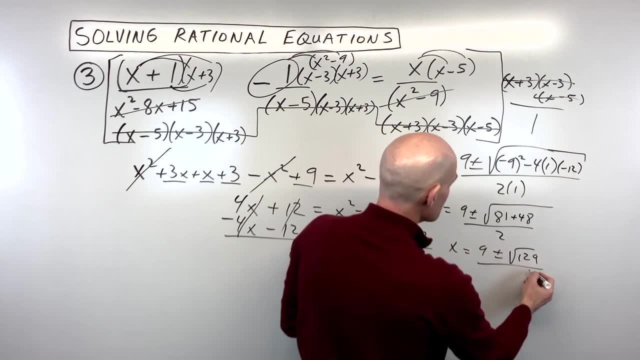 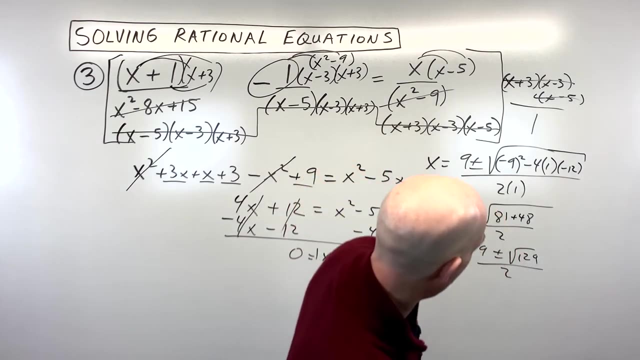 all divided by 2.. And let's simplify this down a little bit more. This comes out to 129, which I don't think can be simplified. I don't think there's any perfect squares you can pull out of there, Is there? Let's see 129,. you could divide that by 3.. Let's see: 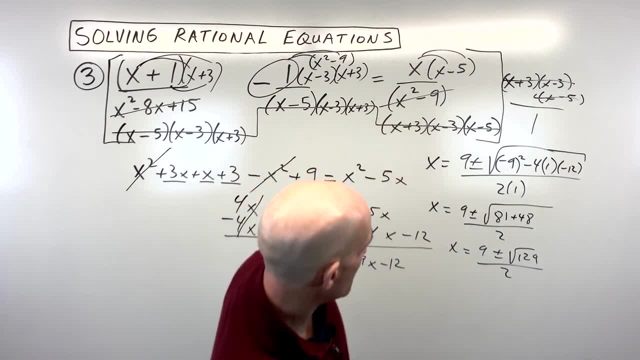 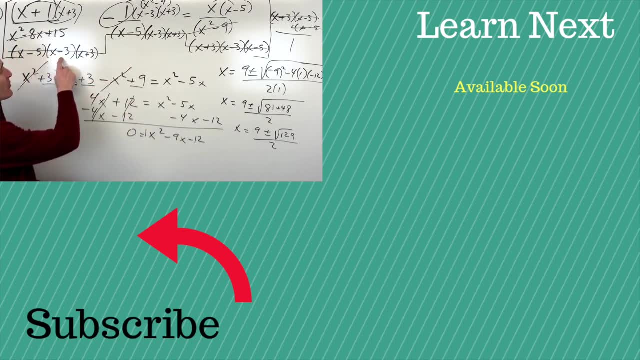 That's 43, but 43 is prime, So it looks like this is as far as you can go, And what we want to watch out for is that you can't divide by 0. So x couldn't be 5,, 3, or negative 3,, which this clearly. 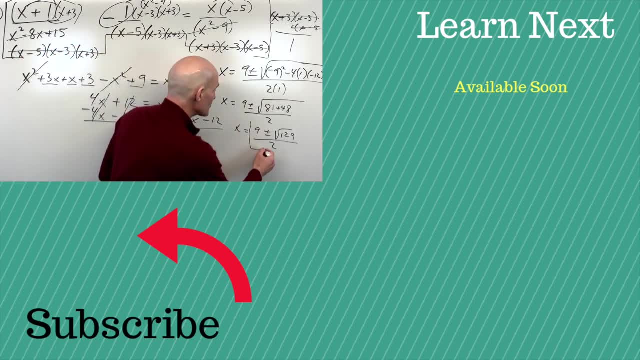 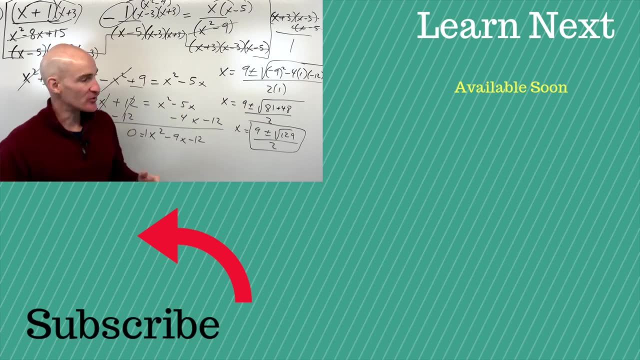 is not, So that would be your final answer. So you've got two solutions here. Great job. If you want some more examples, follow me over to that video right there where we talk about you know, solving more of these rational equations. I'll see you in that video. 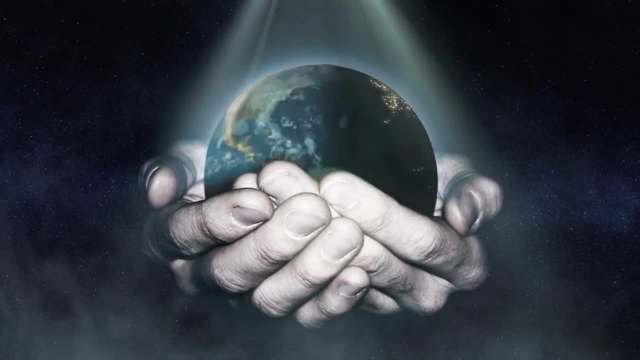 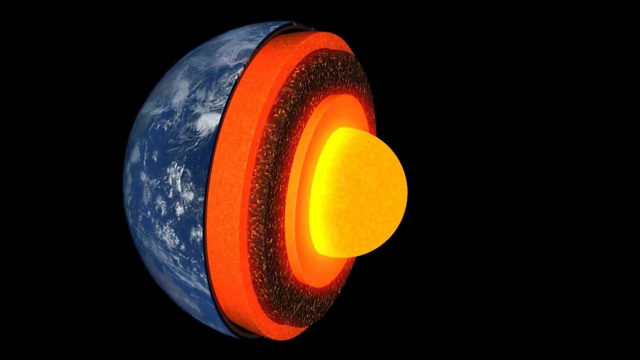 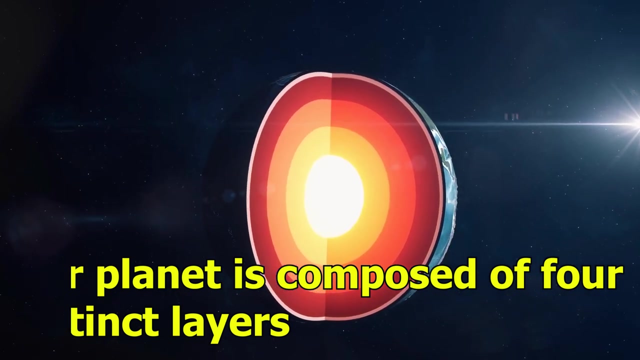 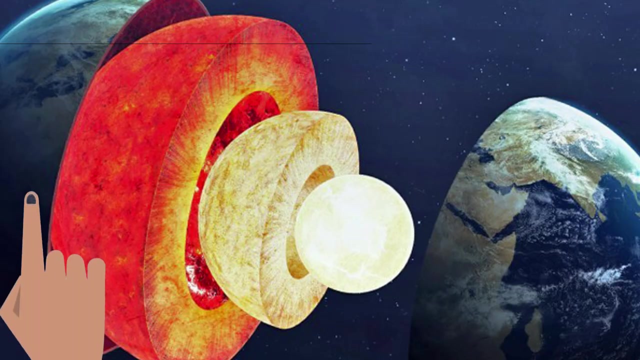 If you could hold the Earth in your hand and slice it in half, you would see that there are different layers to it. Our planet is composed of four distinct layers – crust, mantle core and inner core. Let's understand each layer, starting from the very